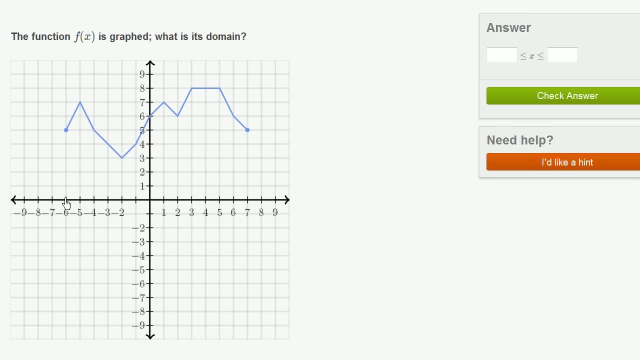 It's not defined for any of these values. It only starts getting defined: at x equals negative 6.. At x equals negative 6, f of x is equal to 5.. And then it keeps getting defined. f of x is defined for x all the way from: x equals negative 6. 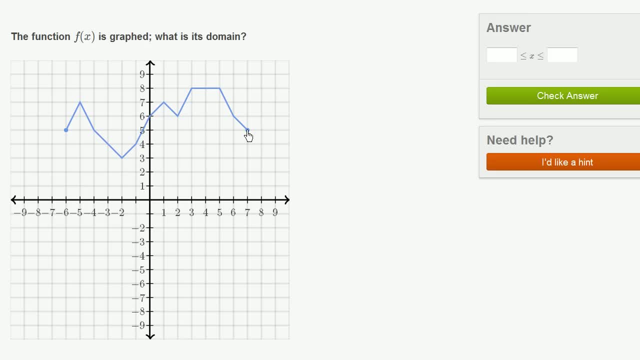 all the way to x equals 7.. When x equals 7, f of x is equal to 5.. You can take any x value between negative 6, including negative 6, and positive 7, including positive 7. And you just have to move up above that number. 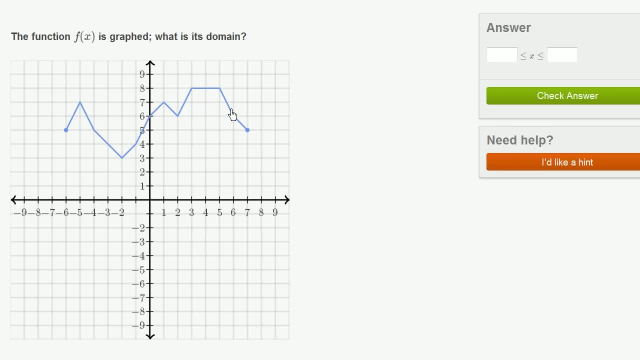 wherever you are to find out what the value of the function is at that point. So, the domain of this function definition. well, f of x is defined for any x that is greater than or equal to negative 6.. Or we could say negative 6 is less than or equal to x, which? 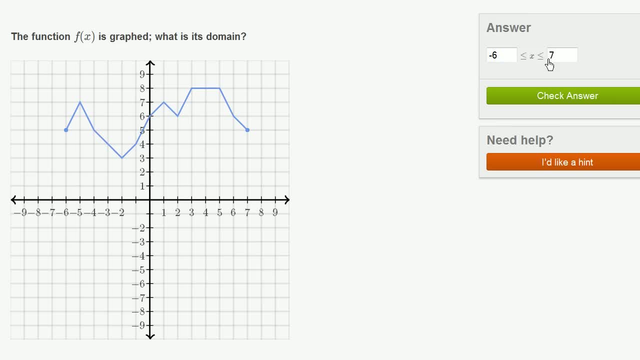 is less than or equal to 7.. If x satisfies this condition, right over here the function is defined, So that's its domain. So let's check our answer. Let's do a few more of these. The function f of x is graphed. 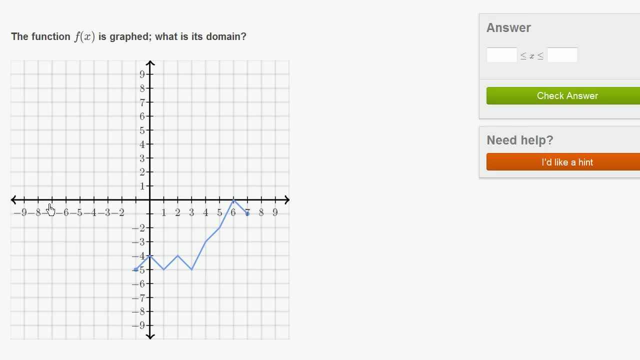 What is its domain? Well, exact similar argument: This function is not defined for x's negative 9, negative 8, all the way down, or all the way up, I should say, to negative 1.. At negative 1, it starts getting defined. 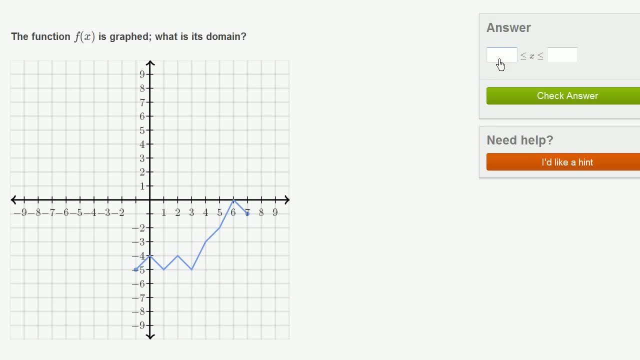 f of negative 1 is negative 5.. So it's defined for negative 1 is less than or equal to x, And it's defined all the way up to x equals 7, including x equals 7.. So this right over here, negative 1. 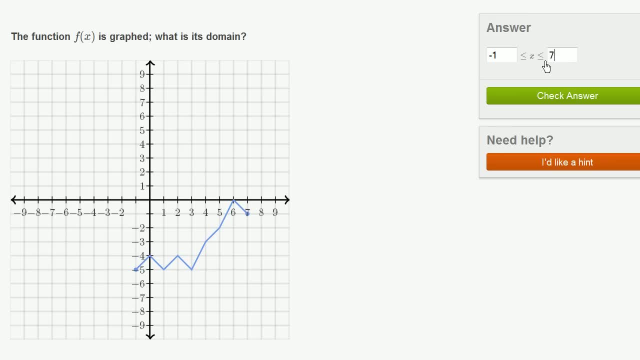 is less than or equal to. x is less than or equal to 7.. The function is defined for any x that satisfies this double inequality. right over here, Let's do a few more. The function f of x is graphed. What is its range? 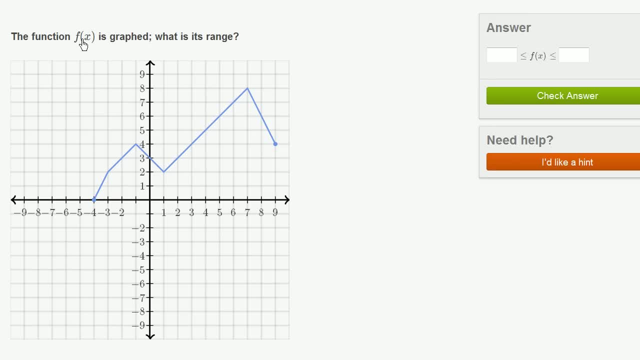 So now we're not thinking about the x's for which this function is defined. We're thinking about the set of y values. Where do all of the y values fall into? Well, let's see The lowest possible y value, or the lowest possible value.